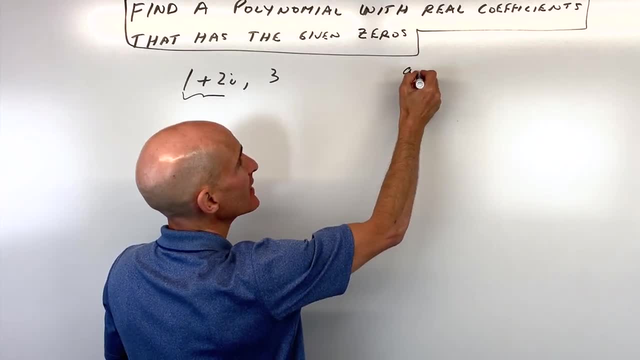 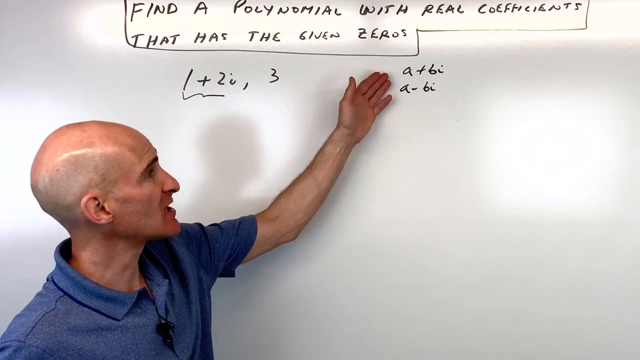 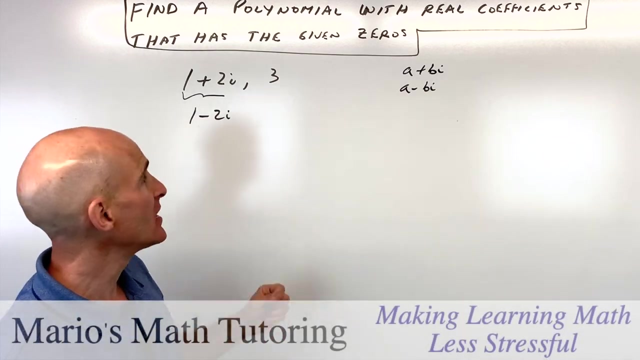 solutions come as conjugate pairs. What I mean by that is like imaginary numbers. in this form, A juntos BI, A minus BI will also be zero. So these come together. so if one plus two i is a zero, we're also going to have one minus two i. So that's part of the trick of this question. The other 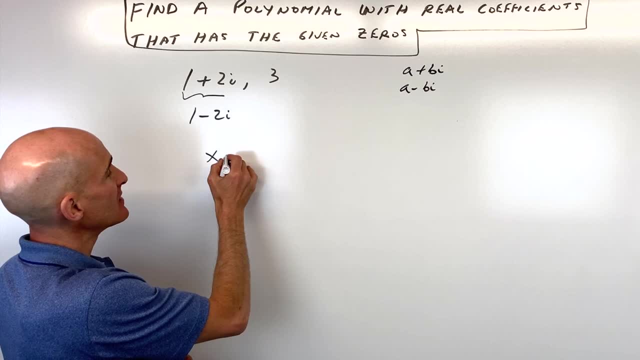 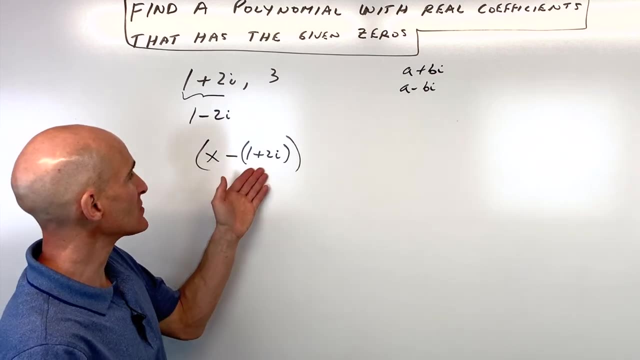 thing is to realize is that when one plus two i is a zero, x minus one plus two i is a factor. So you always have x minus these zeros as factors. so we have x minus one plus two i. we have x minus one minus two i and we have, as Magic has two i. you have a 1 minus two or a minus one minus two i. we also. 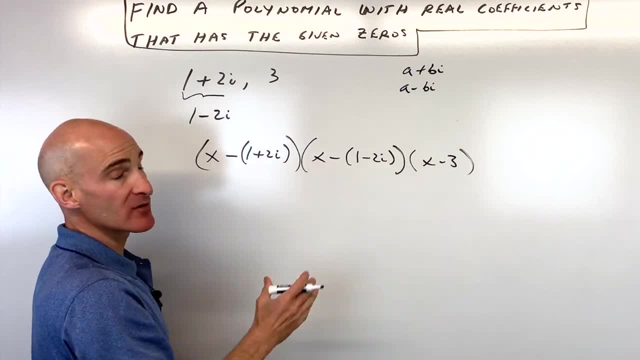 have a 셍 and we have X minus one minus two, and we have: what does that look like in the pixel Chi right now? because the pixel Chi less than zero right now, that's X minus x minus one minus two, I x minus 3.. Okay, so it looks pretty confusing here. How are we going to multiply this together? 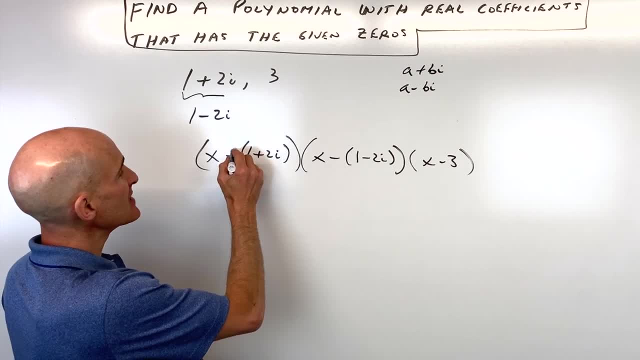 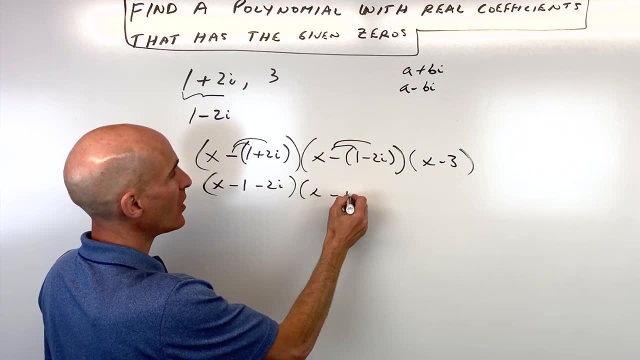 Well, I want to show you a shortcut, And the shortcut is: let's think about distributing this negative in here. So we get x minus 1 minus 2i Over here. we have x minus 1 plus 2i. 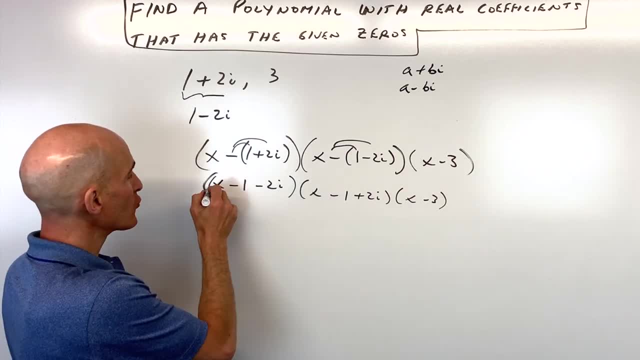 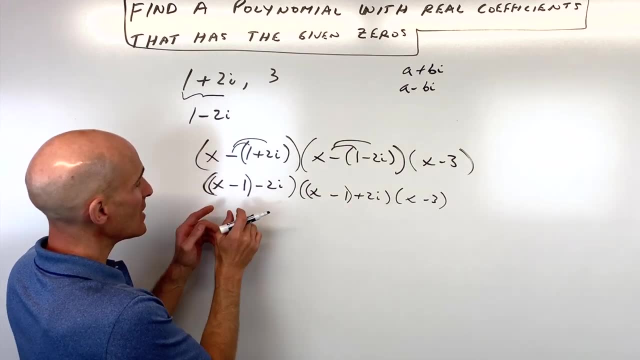 And here we have x minus 3.. So what we can do now is I'm going to group the x minus 1, okay, like that together. Okay, so now we're going to multiply these two groups together first. So if we use the FOIL method, we take this term times this term. We can just think about the. 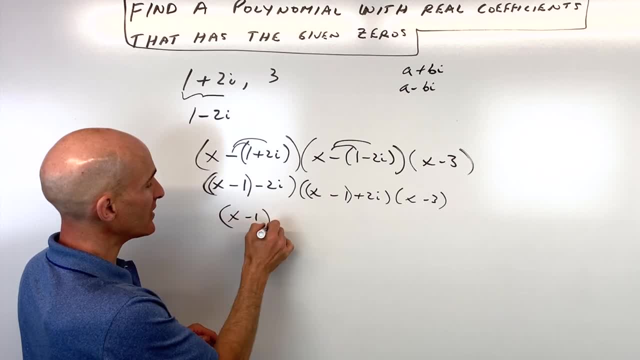 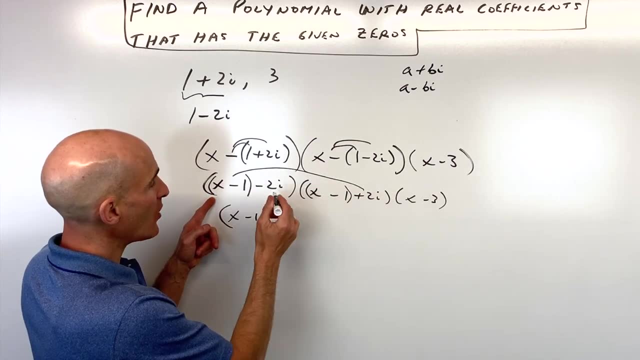 distributive property. This distributed, this is going to give us x minus 1 squared, because x minus 1 times x minus 1.. Now the outside, or if I distribute here, I get x minus 1 times 2i, And if I do the inside, I get x minus 1 times negative 2i, Since 1's positive, 1's negative. 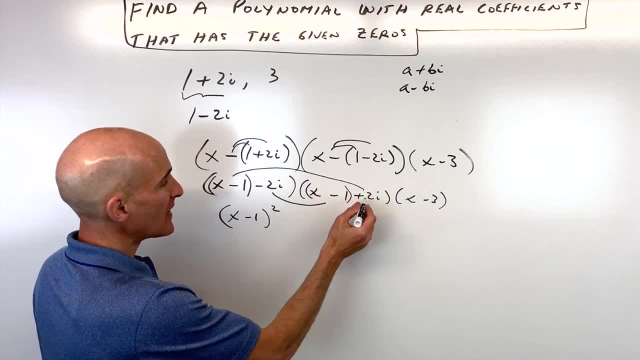 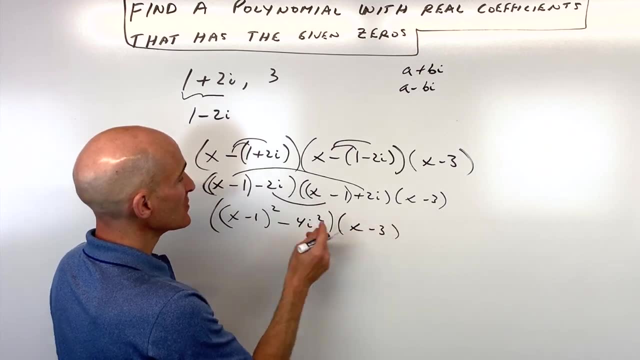 those actually cancel. And then the last terms. we get negative 2i times positive 2i, which is negative 4i squared Okay, and that whole thing is multiplied by the x minus 3.. So this is a nice technique to make it a little bit simpler. So now let's. 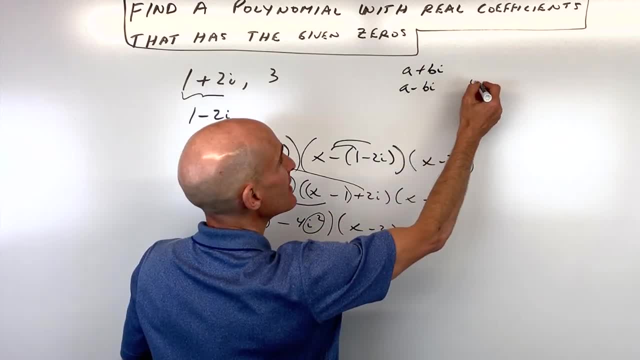 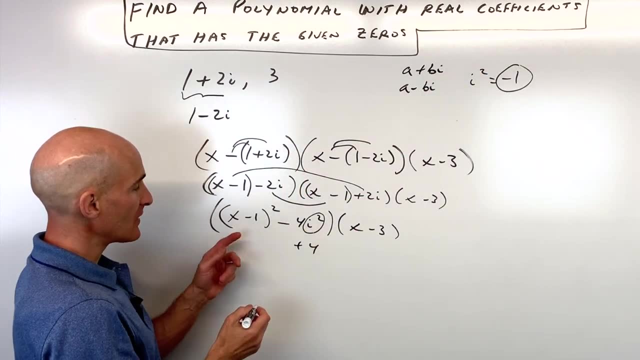 simplify a little bit further. Remember: i squared equals what- This is definitely something you want to memorize- i squared is equal to negative 1.. So we have a negative 1 times a negative 4, which is a positive 4.. If we FOIL out x minus 1 squared, we get x squared minus 2x plus 1..